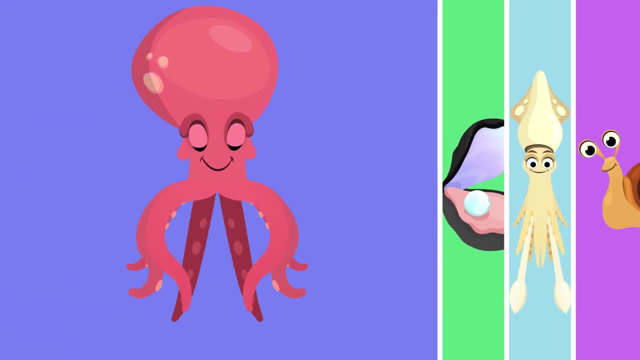 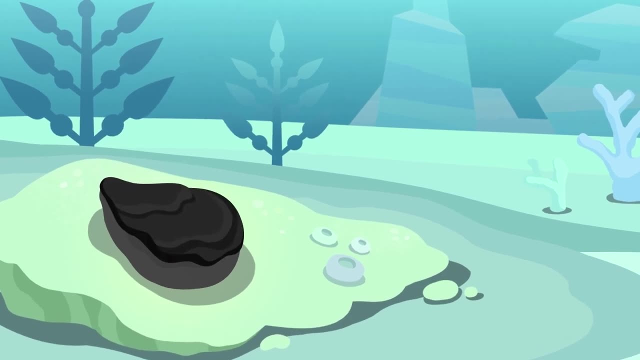 Mollusks. Do you know what kind of animals mollusks are? You don't? No problem, I'll explain it to you. Mollusks are very different from one another, but they also have a lot of things in common. 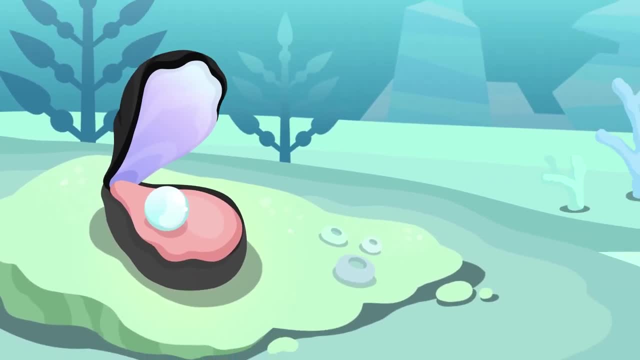 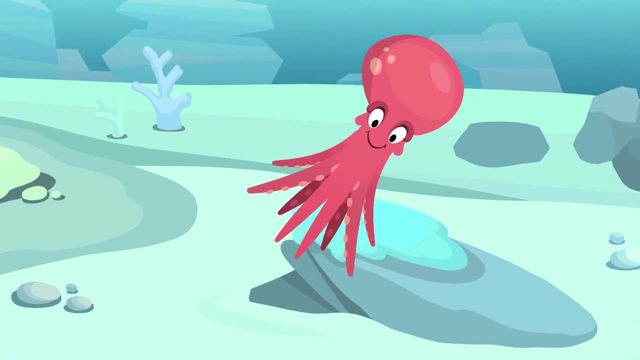 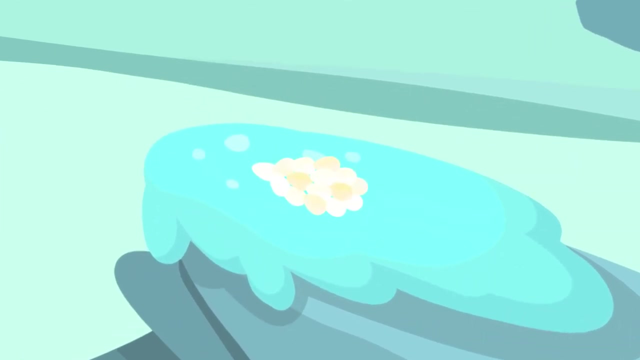 Their body is soft. In some cases it's protected by a shell. In other cases they have no shell at all. Mollusks are oviparous animals. This means they hatch from eggs. Mollusks are classified in three groups. 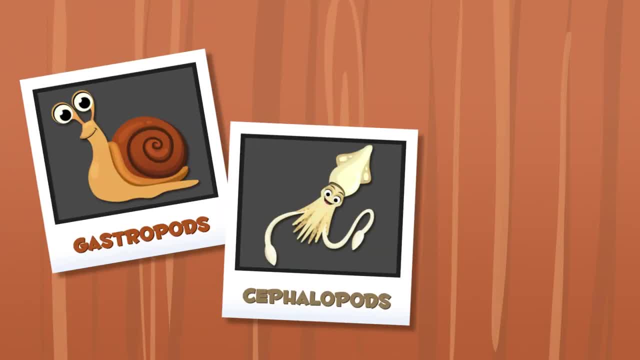 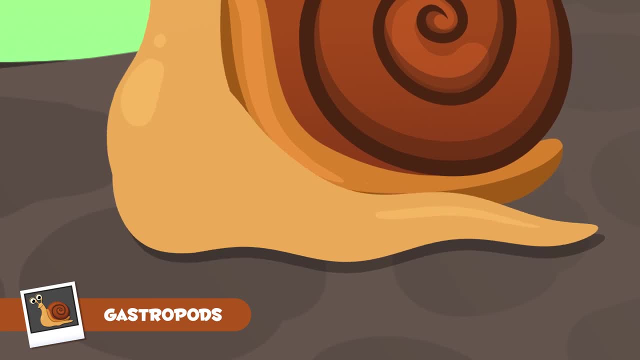 Gastropods, cephalopods and bivalve. We, the gastropods, are mollusks and we move thanks to our muscular foot. Did you know that our eyes are on our tentacles? Snails like me belong to the gastropods group. 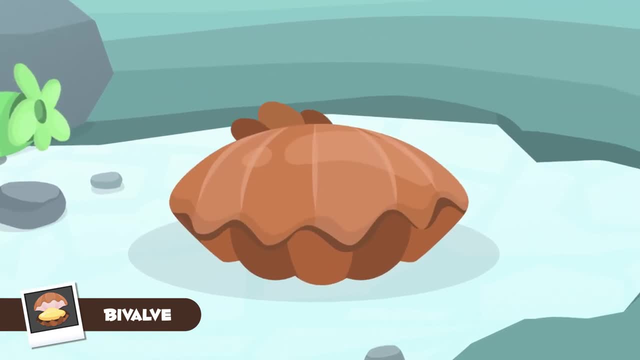 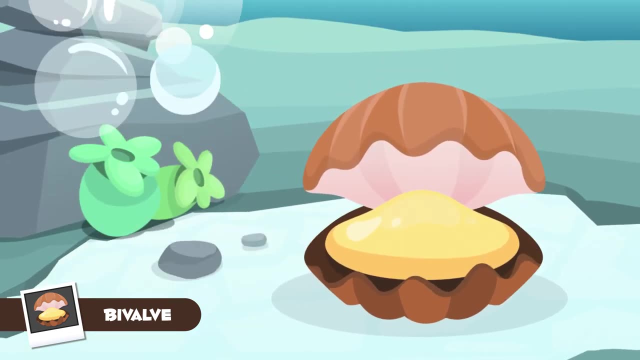 We, the bivalve mollusks, have a shell which closes tightly to protect us from predators. We live in the sea and we are normally attached to rocks or sand. Clowns like me belong to the bivalve mollusks group. 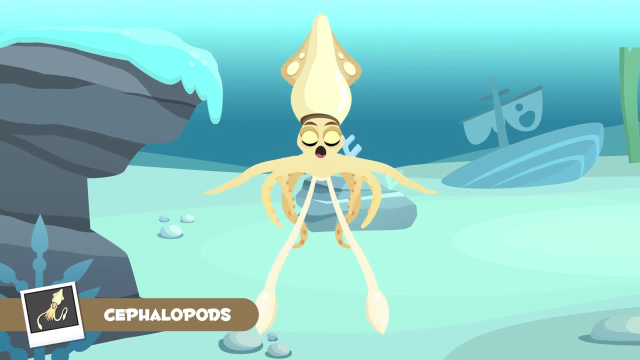 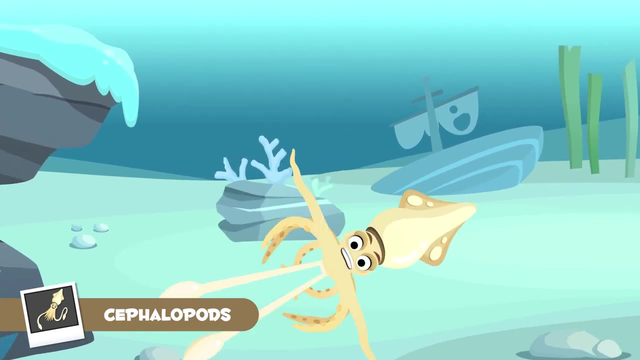 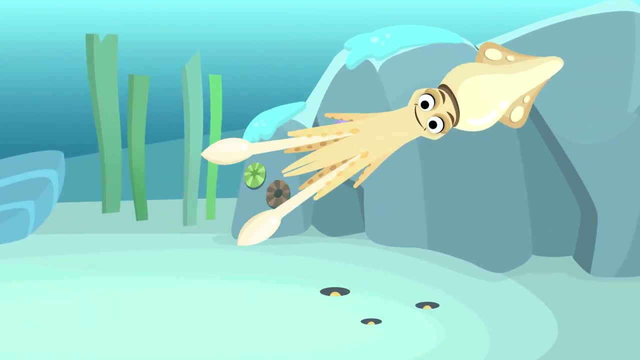 We, the cephalopods, have no shell, but we have long tentacles. We only live in water. Squids like me belong to the cephalopods group. The majority of mollusks, like squids for example, move swimming. 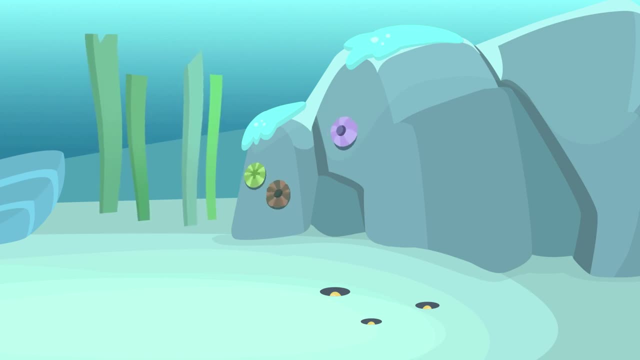 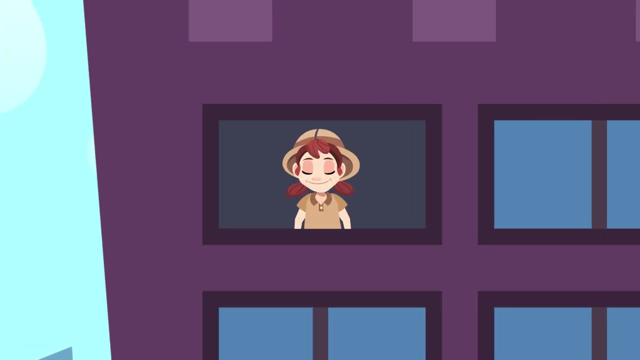 Although there are mollusks like marine limpets that live attached on rocks or razor clams that live on the seabed under the sand, The majority of mollusks, like snails, are mollusks. Did you know there are squids that are as tall as a five-story building? 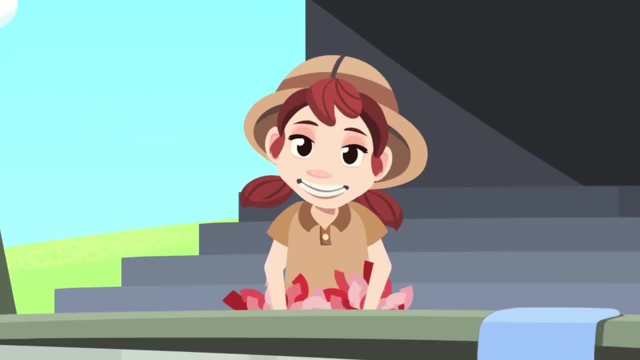 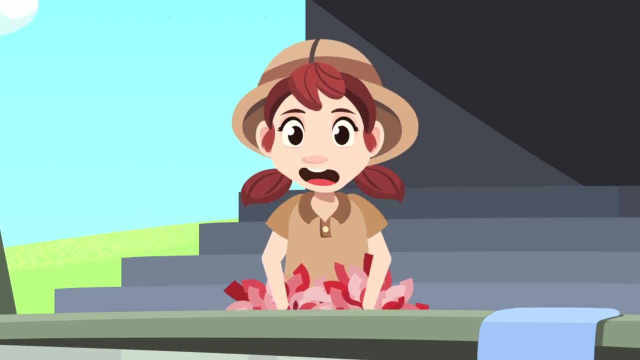 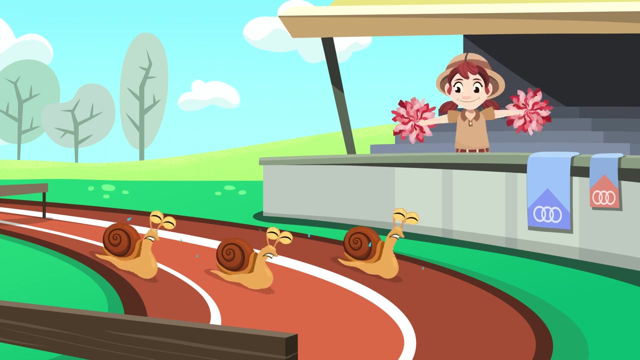 Amazing. Oh no, you're right where I left you. I think that this snail race wasn't a good idea. Well, I'll cheer them up more eagerly, Cheerio. Come on, guys, move along Faster, faster you can do this. 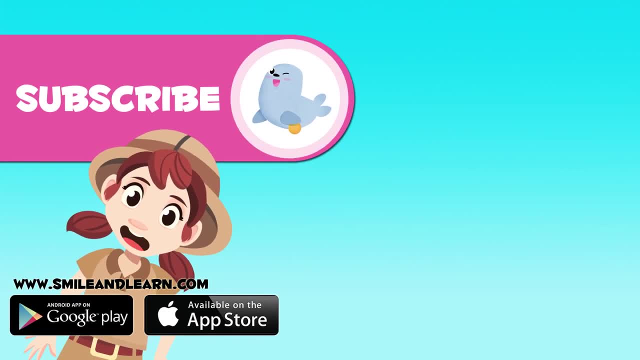 Could you name three mollusks that are not in this video? Leave a comment below and tell us about it. Will you get it right? Oh, to watch more videos, click on the seal and subscribe to our YouTube channel. Stay tuned and don't miss out on the new adventures.